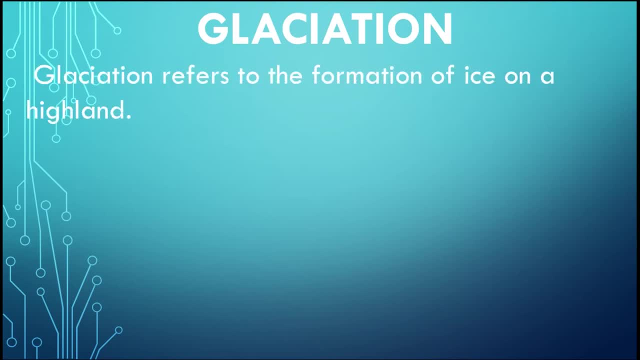 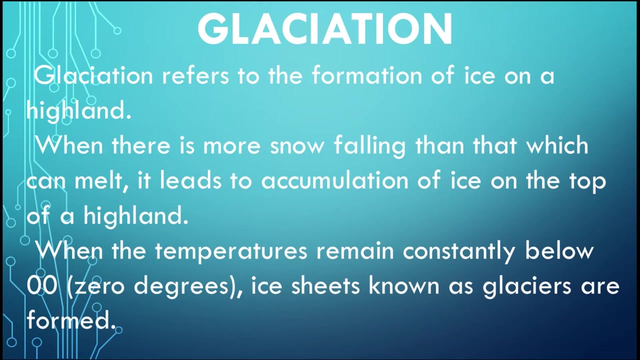 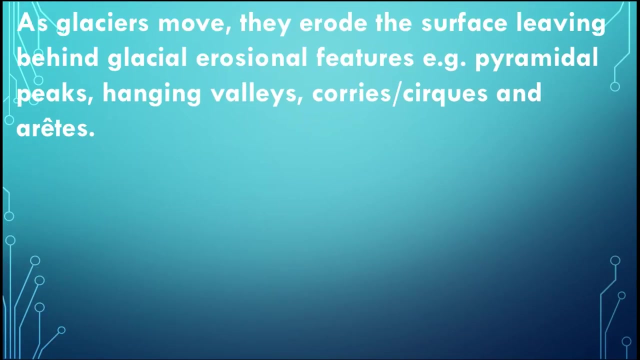 So what is glaciation? Glaciation refers to the formation of a formation of ice on a highland, when there is more snow falling than what and which can melt. actually, It is the accumulation of ice on top of these islands, and then, when the temperatures remain constantly below zero degrees- Actually, they even move to negative degrees- Ice sheets, known as glaciers, are formed. We are yet to understand what glaciers are. So, as we move on, we are saying here that as glaciers move, they 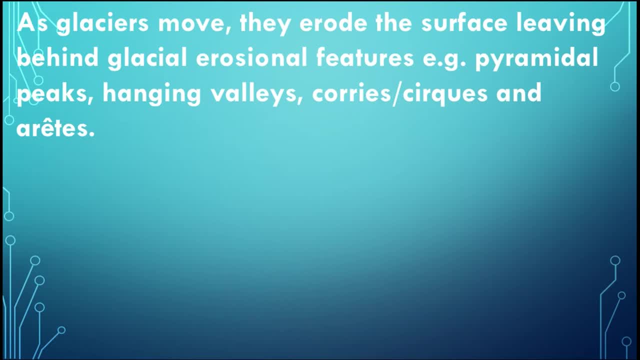 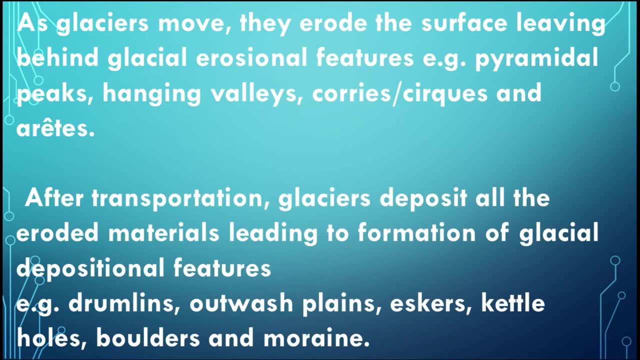 erode the surface, leaving behind glacial erosion futures, for example, the Pyramidal peaks, hanging valleys, Corals, Succuse, ande are rates or so after transportation. Galaxes depot all the rodent materials leading to formation of glacial deposition materials or futures. For example, here we have the drumlines. 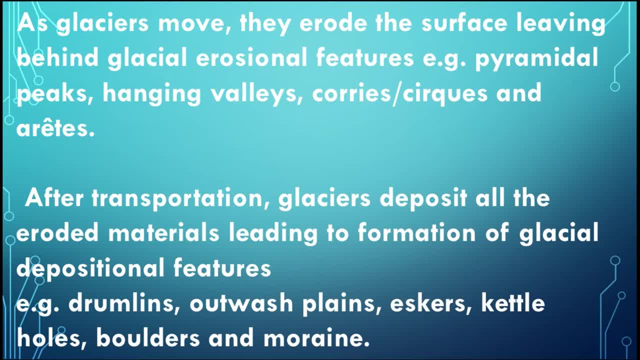 These are examples of the futures formed. when are the glacier deposited materials? we have the outwash planes, We have the eskers and we have the kettle holes, We have the boulders and then moraine. These are formed after the deposition of the glacier. 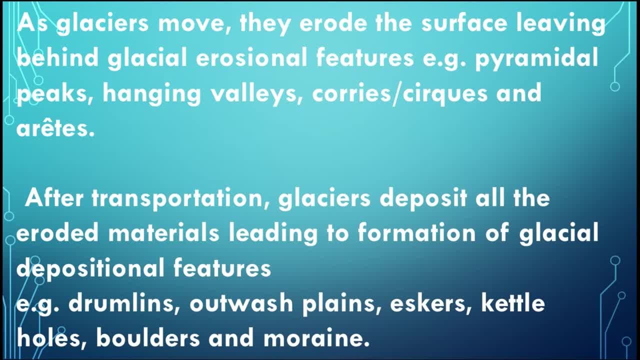 So we are saying the glacier performs two processes: It erodes when it is moving from upslope down the slope, Retreating. it erodes Then later it deposits. So we have what we call the glacial erosion features, The ones we have looked at, the ones up, these ones here. 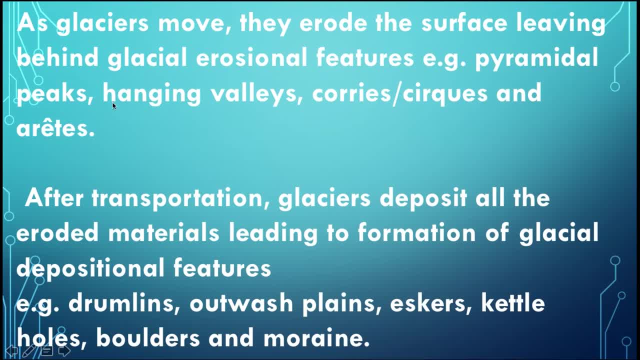 These ones here. So the pyramidal peaks, hanging valleys, corals and circuits and arids are known as glacial erosion features. Then we come to the outwash plains and eskers and kettle holes, and then boulders and moraine. 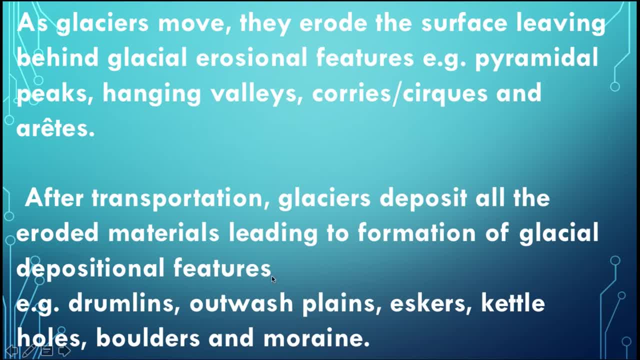 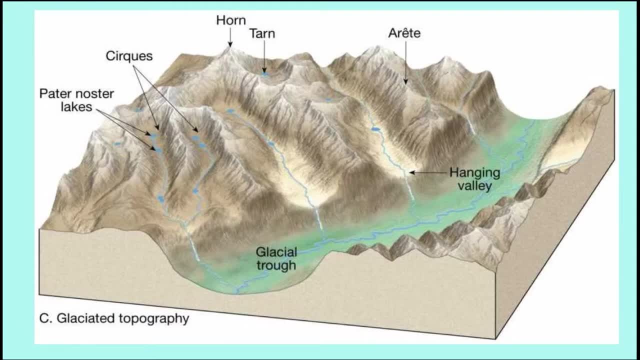 These are known as deposition of glacial art features. We move on. So what we see right here? We are going to start with The erosion features. We see the circuits, We see the hole in which is known as the pyramidal peak. 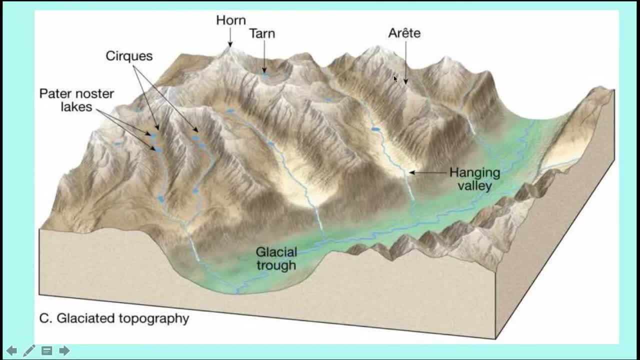 We see the tarn here, Then we see the arids, The knife edge shape, And then we also see the circuits around this area. Then we also see the glacial troughs, The hanging valleys here, And we shall move into detail to see what this. 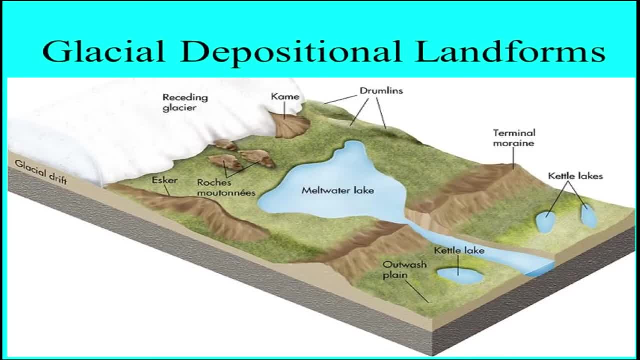 And then, when we move down here, We see what we call the glacial depositional landforms, Where we have the drum lines, These ones. here We have the calm, We have the receding glacial Which is actually coming down here. 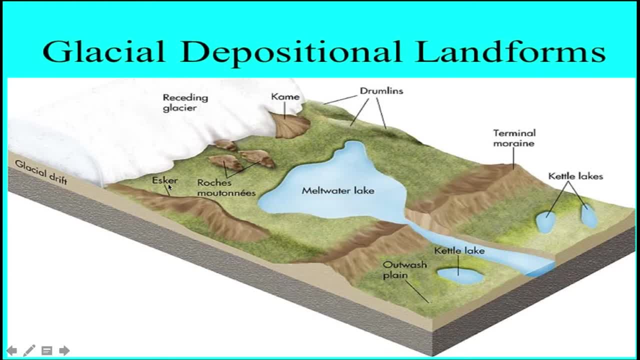 That forms all these features. Then we have the eskers, We have the kettle And then we also have the terminal marine around these areas. So these are features that are formed due to the glacial depositional process, When the glacial deposits certain materials there. 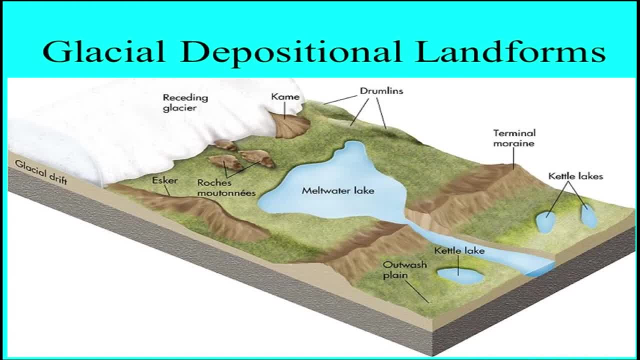 It is the formation of these features that we are looking at right now. so the factors that are quite limiting glaciation in east africa, and we have quite a number here. we have what we call altitude, uh, height above sea level, as we have talked earlier, that in east africa we only have glaciation in few kind of areas because of the height. 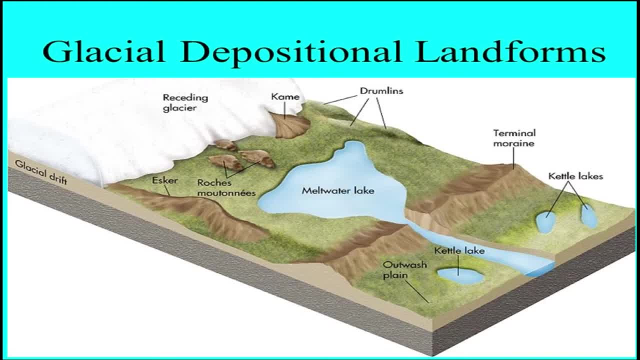 the two above sea level, for example, only have it around the highest peaks. and then why is this so? because the higher you go, the cooler it becomes. as you move up, you lose a degree of temperature as you move up, so we also have latitude. uh, we lie across the equator and definitely we have. 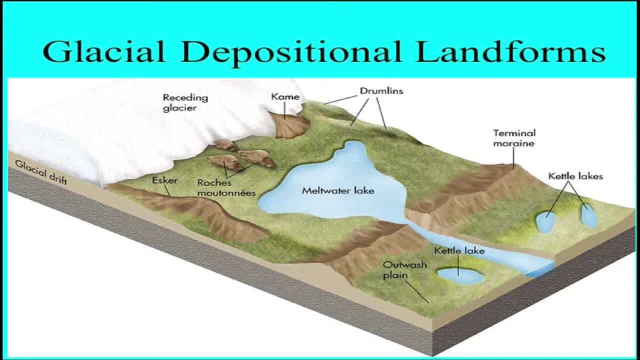 quite hot temperatures around this area, limiting glaciation. uh, these are factors that are limiting glaciation in east africa. a factor number two: we can look at global warming. uh, it's increasing, actually, the temperatures are increasing. and then we also have another factor known as low precipitation. uh, definitely, we have quite 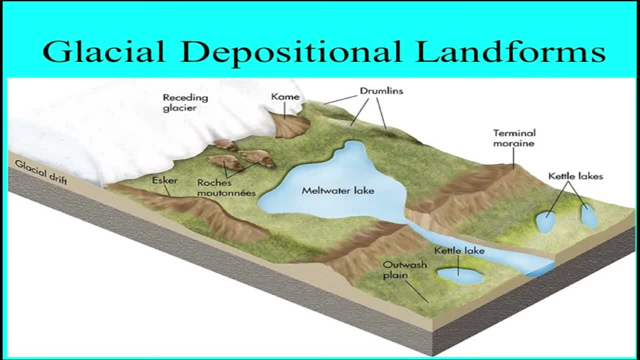 low precipitation around this area of east africa and then expansion of the deserts. you know, up north we have the sahara desert that is expanding southwards and this limits glaciation. remember, glaciation is where we see snow falling for quite a long time, accumulating, forming ice sheet which 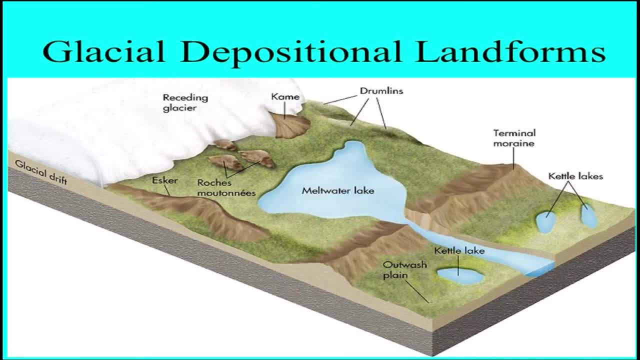 is a glacier and definitely that is during cold condition, degrees falling below zero. but when now temperatures are increasing, definitely we can't see snow falling and accumulating, forming a glacier. we also have another factor known as industrialization. this increases temperatures. we also have urbanization. we have the the rain shadow effect. 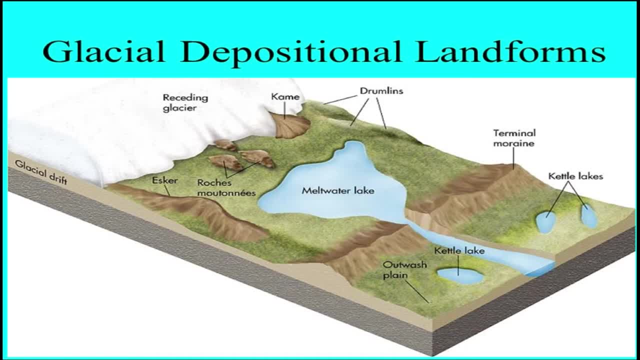 all these factors explain why we see limitation of glaciation in east africa. then we also look at the functions of glaciation east africa. we have quite a number of them as we move into this study today. uh, once to our attraction, we see people coming in and we see people coming in and we see 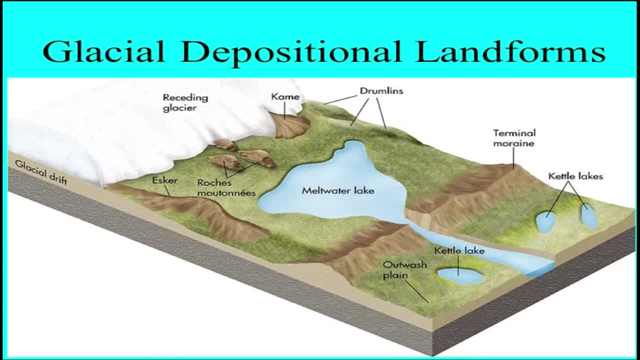 people coming in the hanging valleys from waterfalls which are used a source of water for rivers, for example, uh on the mount of mount rinzori, where we have the mubuku river, which is important for irrigation, and then we have the whitewash plains, which provide fertile land soils for agriculture. 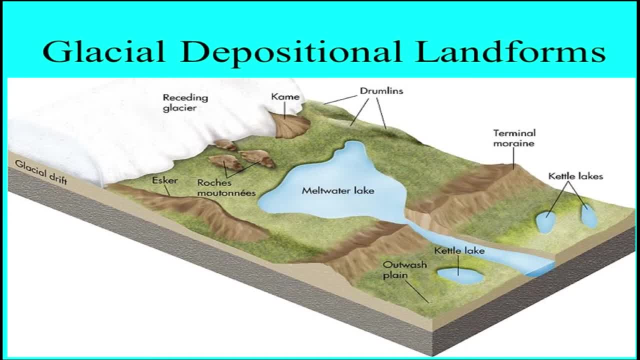 then also research and study purpose. right now we are in study- uh, that's how important they are, study and research purpose, and in many others, those are the pros over our topic today. there are also good sites for filming and photography that are quite amazing, as we shall see then. the cones, or the problems, or the 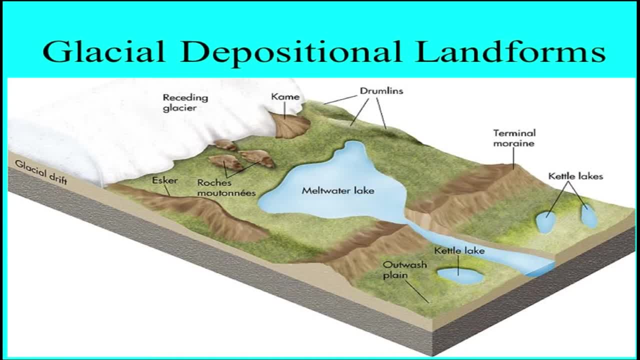 demands that we have around this area is that they form rugged terrains which are not good for a kind of transportation and human settlement. also, the temperatures here fall below zero, which are quite not good for human settlement. so allow us dive into it more and we look at what a glacier is. 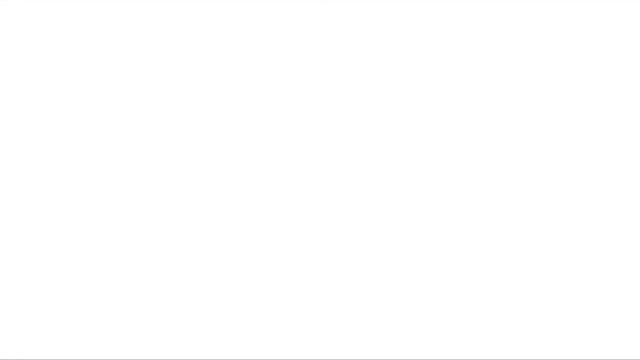 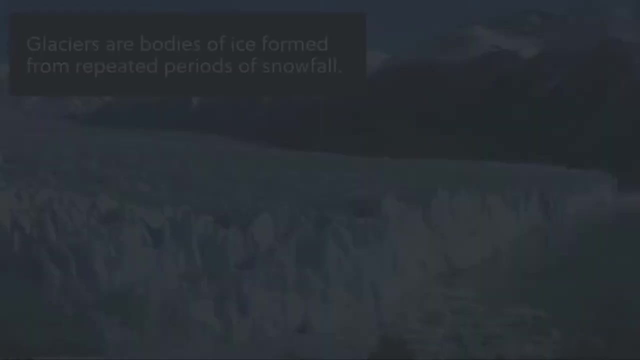 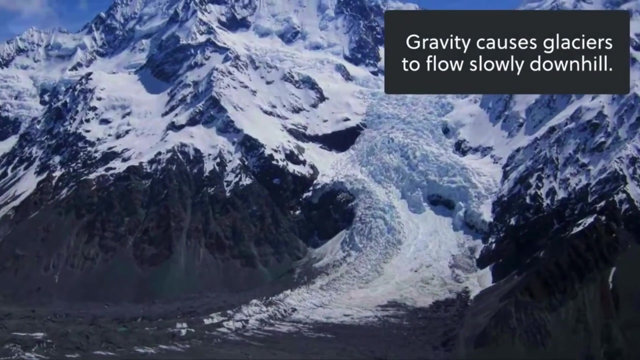 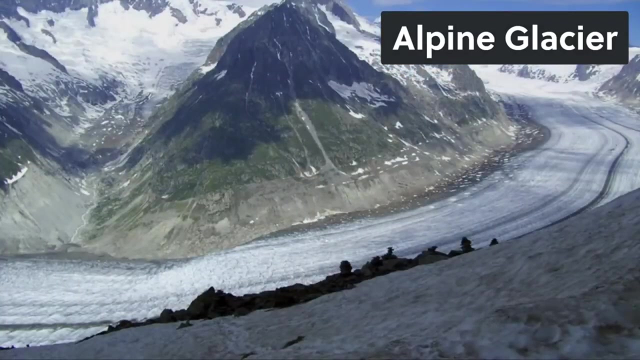 and how a glacier is formed. so let's understand what glaciers are glaciers? what are glasses? that's a good question to ask ourselves. so we are saying glaciers are bodies of ice formed from repeated periods of snowfall. due to gravity, glaciers are forced to move slowly down the hill. definitely, we have different types of glaciers, for example, the alpine. 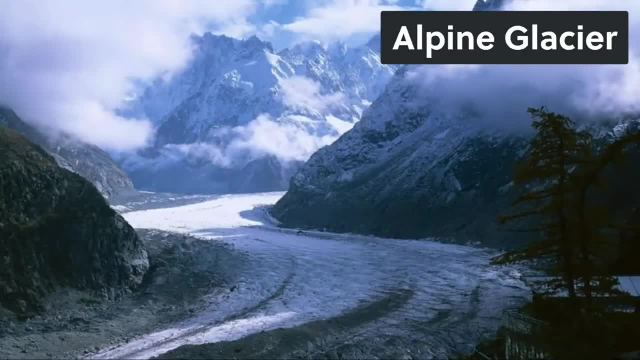 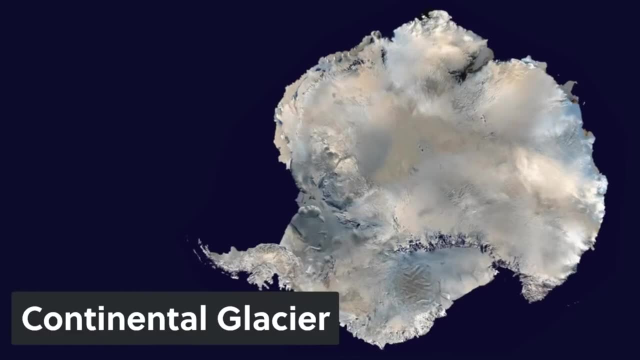 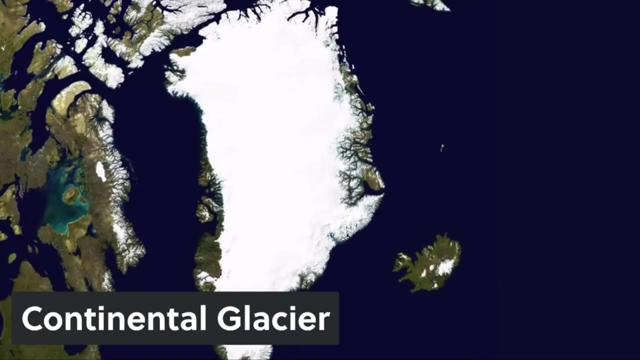 glacier. this is formed in mountain areas. then we also have what we call the continental glacier is a massive glacier that actually moves from the, the center, having actually the bigger land, and moving outwards from the center, for example in the antarctica and then also in the greenland. 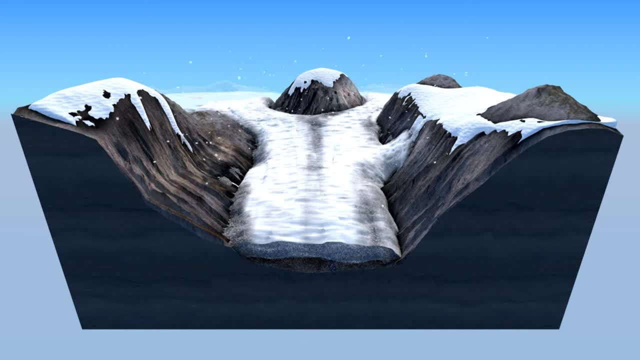 areas where we have the continental kind of glacier. so how is? how are these glaciers formed right here i want to look at how they are formed, winter season or cold conditions. during the period of cold conditions and winter, we have said, snow falls for quite a long period of time. 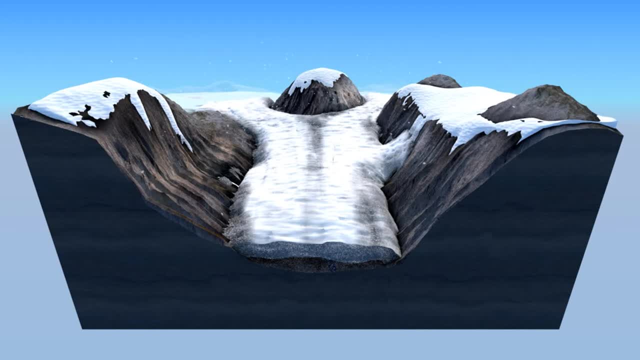 and, with the time, it accumulates, forming a large ice or a large boot of ice, due to the repeated periods of snowfall. so what we are seeing down here is that snow is falling over and over over period of time, accumulating, forming what we call an ice sheet, which is referred to as a glacier. 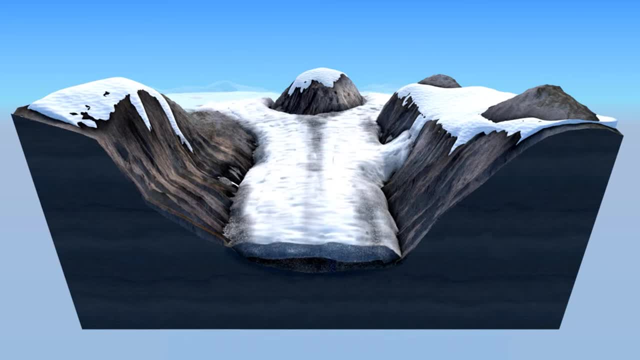 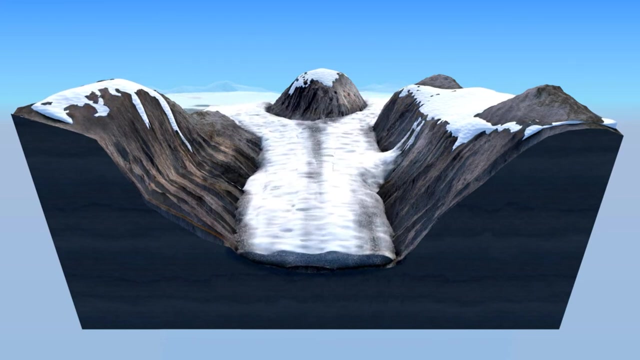 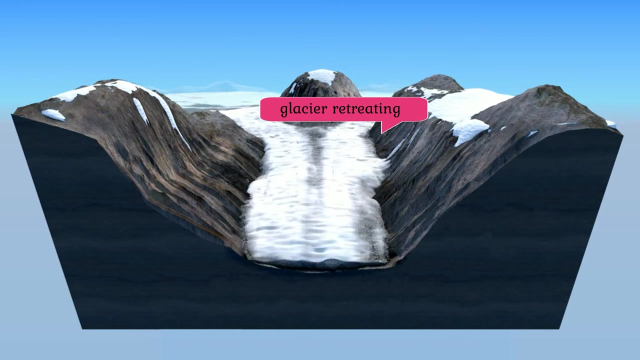 so, during summer seasons, this ice is forced to melt due to the pressure that is above, and then it starts to retreat down the hill. as it is retreating, the glass has performed two processes: one it erodes and then deposits. then, when it is eroding, we are going to see certain 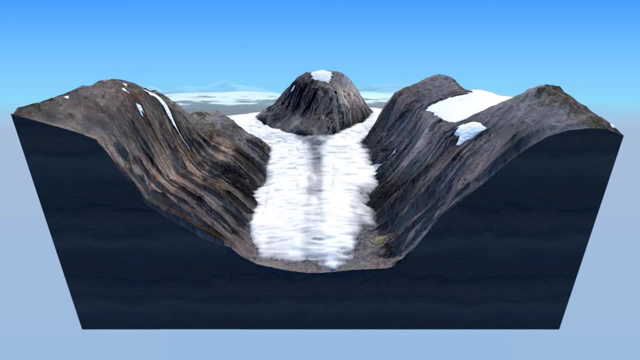 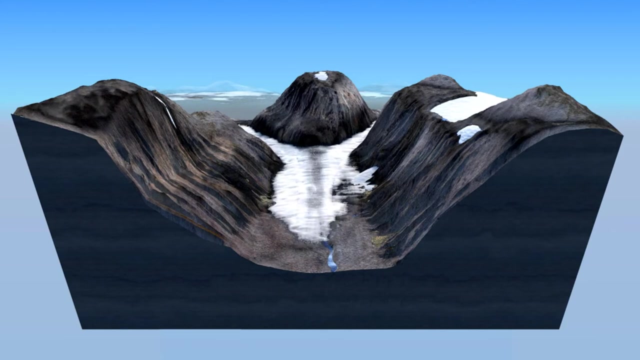 are formed already. we have seen them earlier. so what do we see right now? it is literally eating as it is melting down due to the hot conditions. as it is it treating, it forms what we call the alluvial funds later around that area. so this retreating happens over time due to the hot kind. 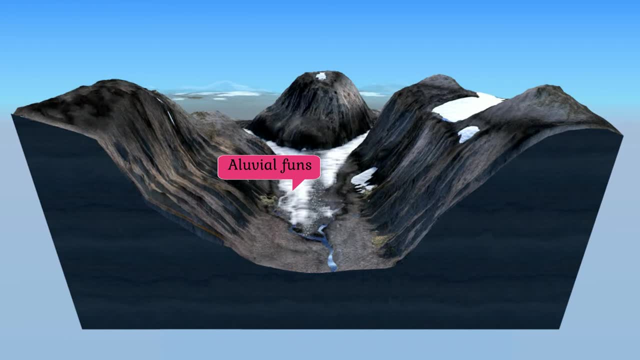 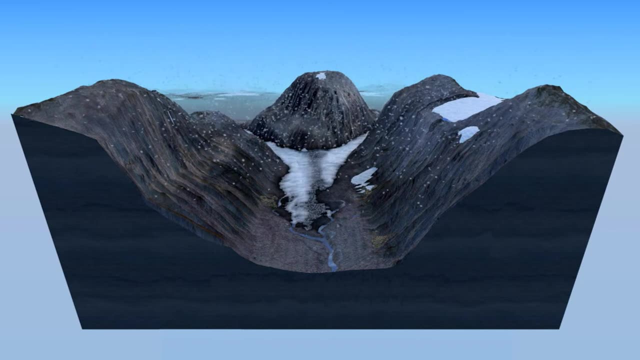 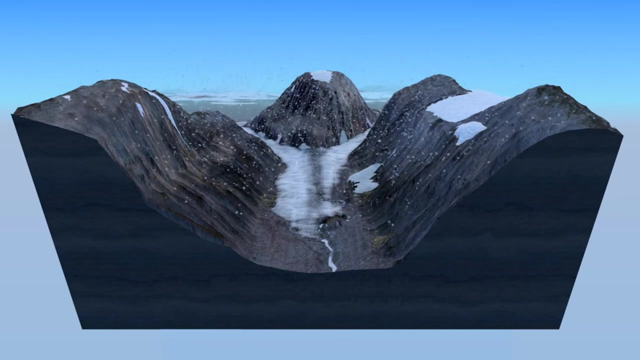 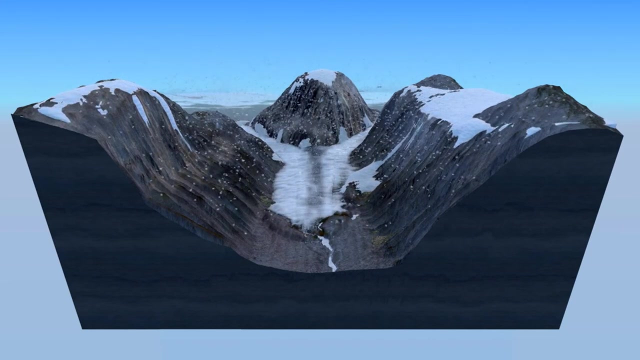 of temperatures with the time. later on, the conditions come again, the cold conditions. then we again see snow falling as it is. as it falls over again, we see accumulation of the snow time after time. with time it again forms a glacier. when these glasses are formed again, they accumulate and then occupy the mountain tops. 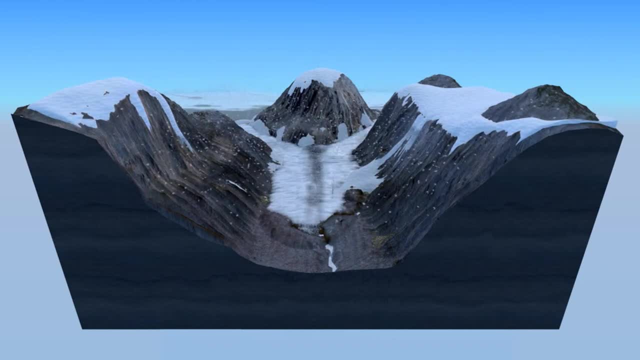 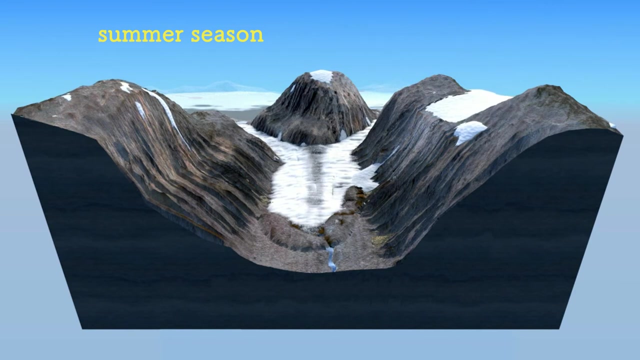 you can see up here and then the valley tops, and then within the bottom of the valley, uh, in deformation. later they will do the same processes that we have talked about. now, when summer season kicks in, we are going to see the same thing happening here. now we see again ice melting and it is melting. 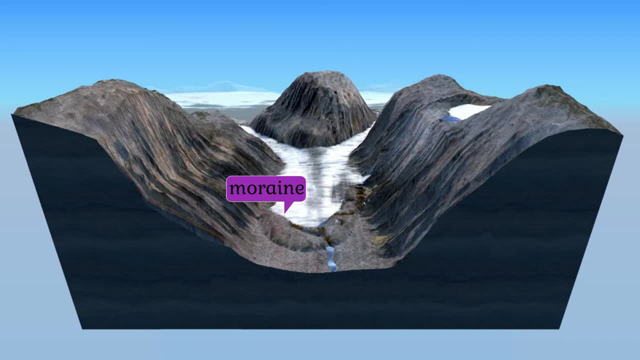 it is literally hence leaving the deposited material, which was called moraine, around the bottom of the valley down the slope. so with the time it again forms what we see as rivers around this area, and then the hanging valleys up there where we see a turn. it again forms a lake up there and then water starts to flow. 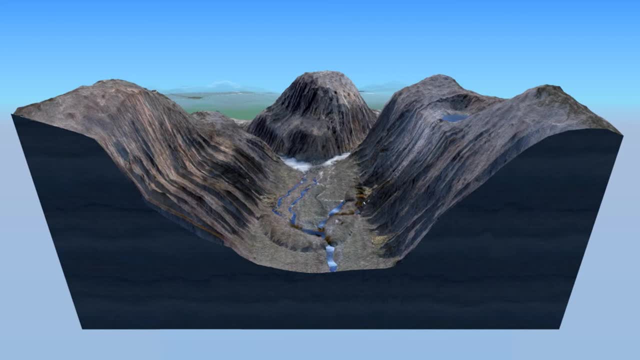 and where does this water come from? it is as simple as melting ice. that produces this water, and actually glaciers are one of the number one uh uh futures that form the fresh water on planet earth. with the time, the the valleys tend to grow, the vegetation time, and then we see rivers being 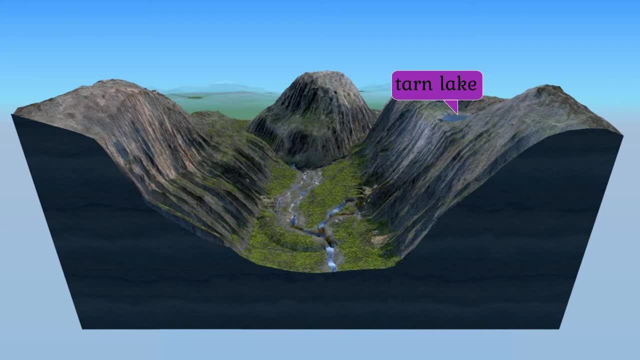 formed and lakes. in the town, in the hanging valley, we see kind of u-shaped formation of valleys and then we see a vegetation growing and even later trees come up. so this is the process that leads to the formation of these clashes and then with the time they do their two processes, that is. 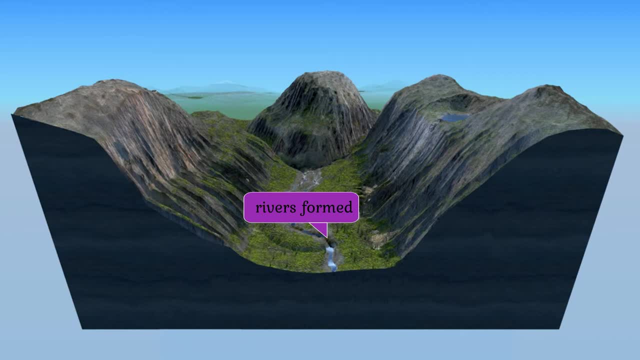 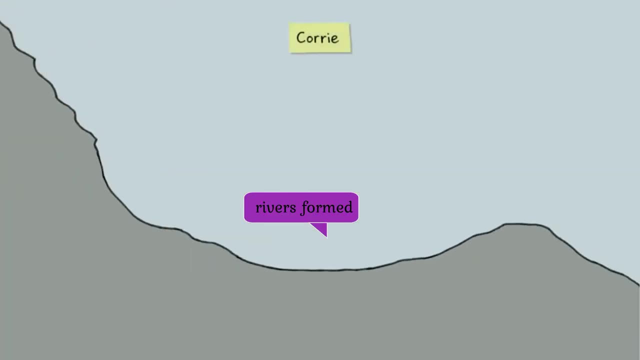 erosion and the deposition. so what? move on and look at these other futures formed and how are they formed. for example, right now we are looking what we call a core coreys are formed when, again, the snow accumulates and fills up a cavity within the mountain. these cores later fill up and then this: 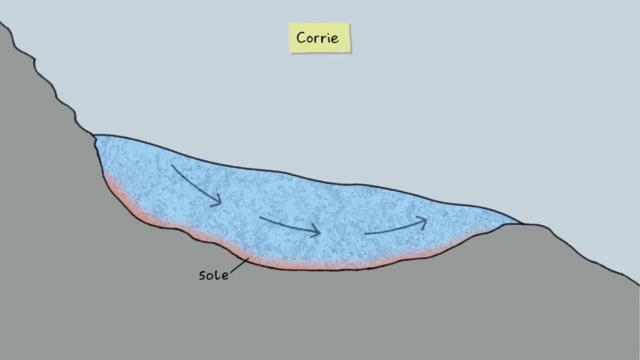 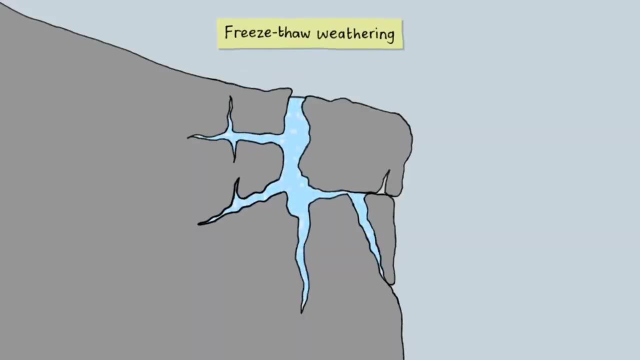 glacier that is formed within the depression due to the weight, is forced to move in the process known as the rotational slip. with time we see the freezing thought weathering up the mountain, where water fills up the cracks of the rocks and then freezes and expands, freezes and expands. 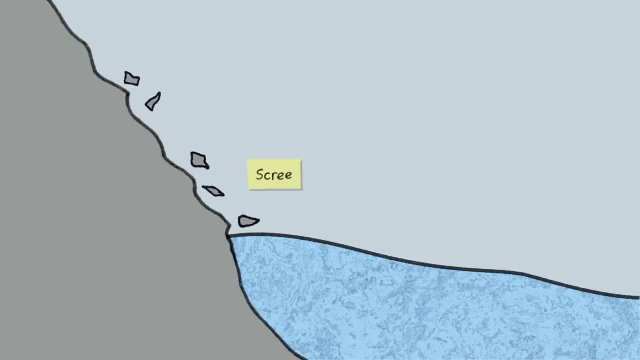 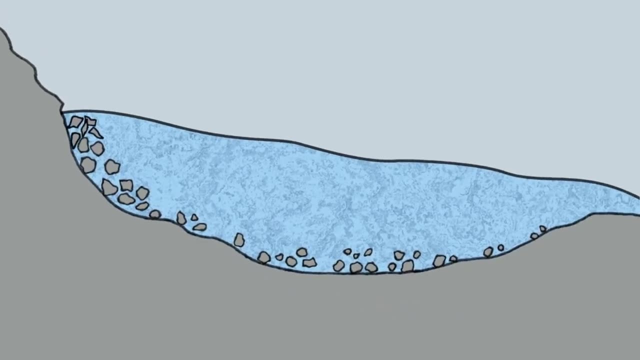 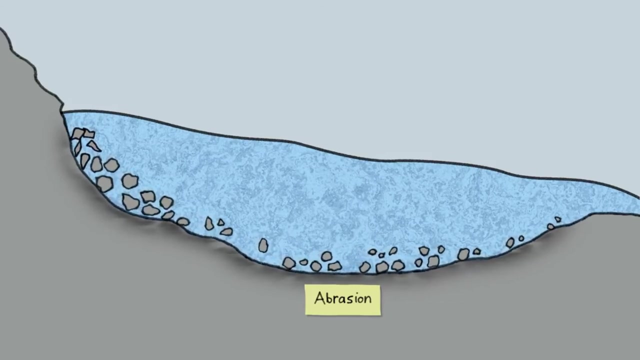 as it is expanding, it leads to disintegration of these rocks. they fall into this big glacier And then go beneath the glacier. And as the glacier is moving down, it causes erosion in a process known as abrasion, where these now crack the surface. 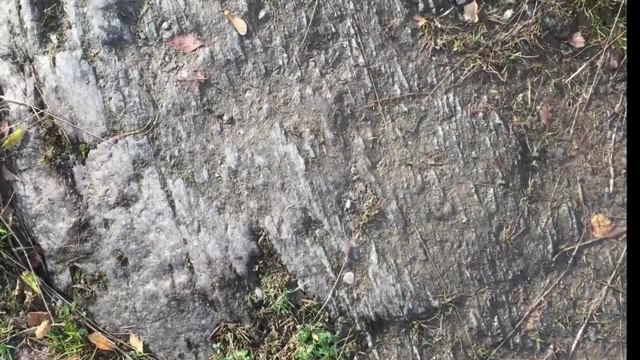 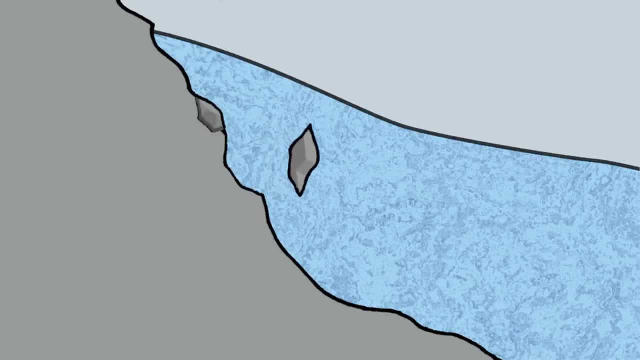 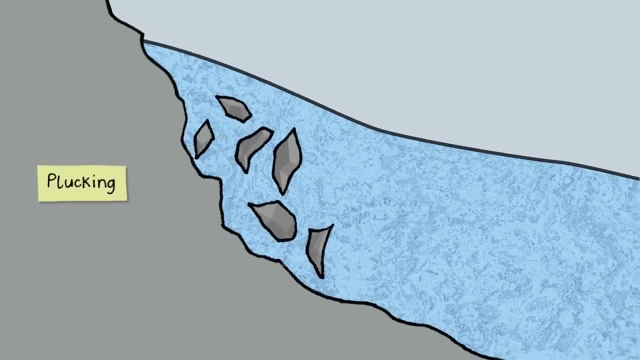 I think you can see in this now They have already cracked and smoothened that surface as they move down the slope, So that's known as abrasion process. Then also with time, this glacier that is heavy in weight, it causes what we call plucking. 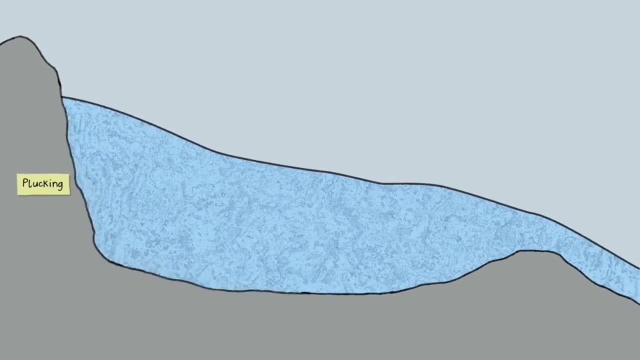 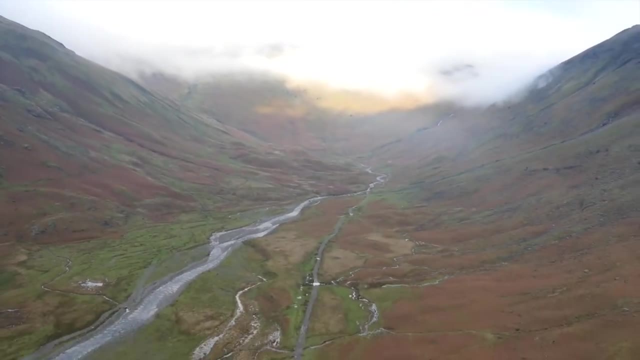 That's another process of erosion. It plucks off the massive boulders of rocks, hence forming what we call a tarn one we see there. So in this valley that we see right now, it has also formed what we call a U-shaped valley. 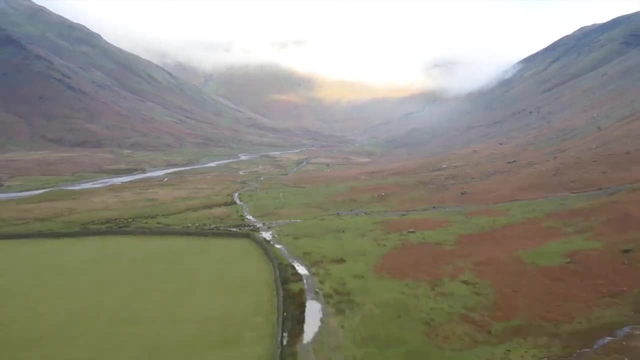 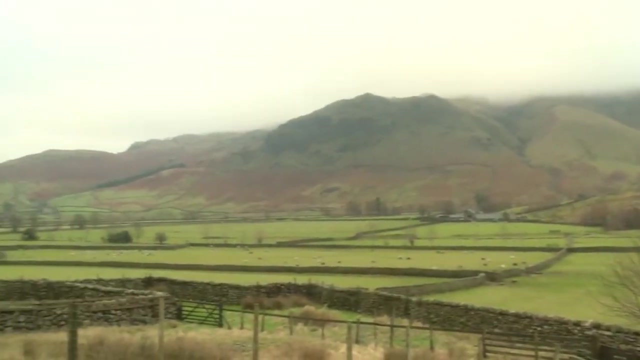 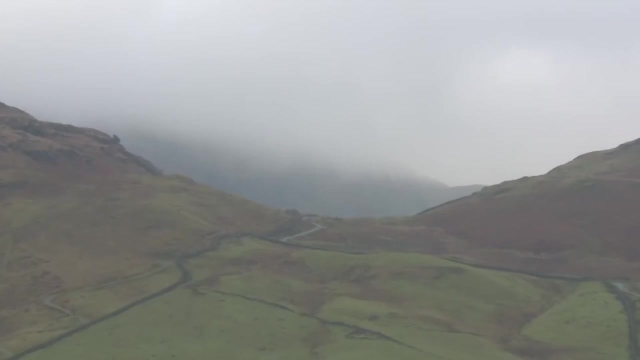 due to its erosion, that is coming from up the hill, down the hill, forming what we call a U-shaped valley. Okay, What we see here that's some time back due to the process of water glaciation. So what we see is a hanging valley which was formed by that simple glacier. 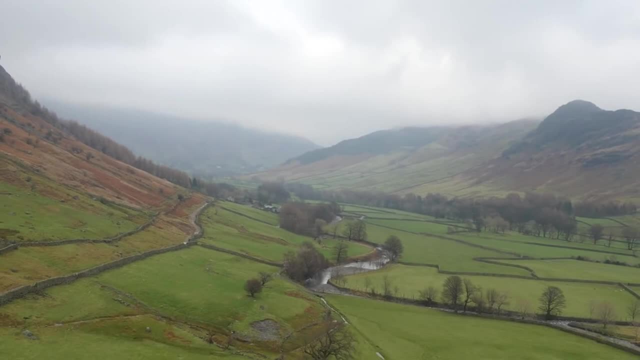 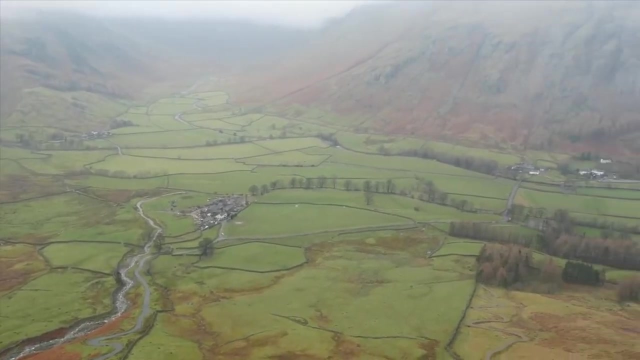 that was unable to erode down the slope, Then from that also what we call the interlocking spars, which are formed by the retreating of this glacier, and then the truncated spar up into the hills. What we see here is a smooth valley. 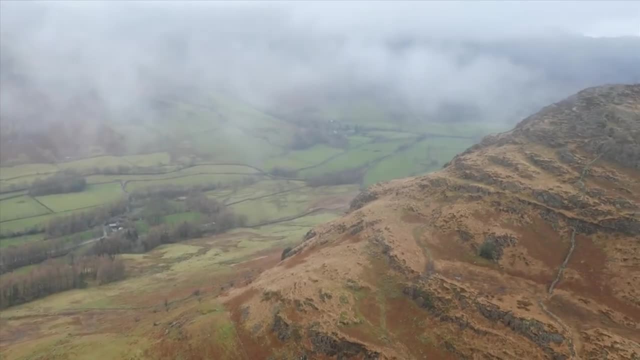 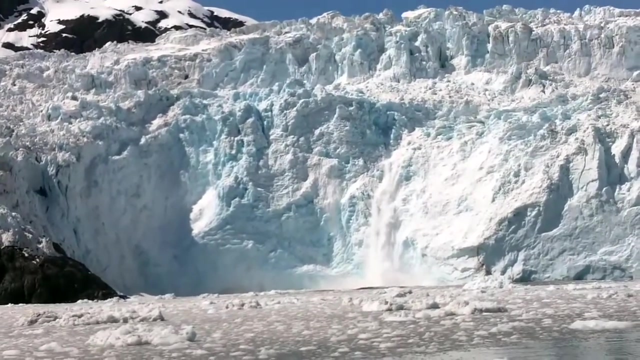 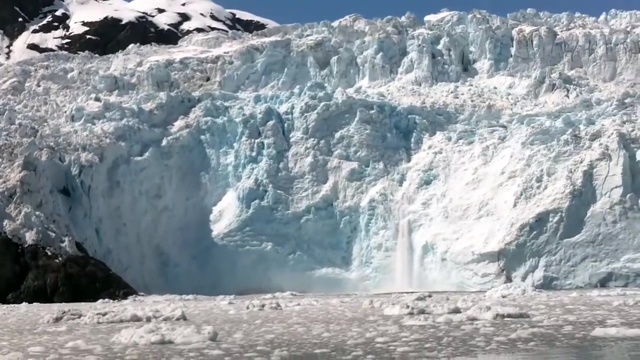 which was formed due to glaciation. Yes, right now we see how this glacier moves and retreats down the slope. Right we can see there is a glacier and ice on the mountain And with the hot conditions and the weight of this glacier, 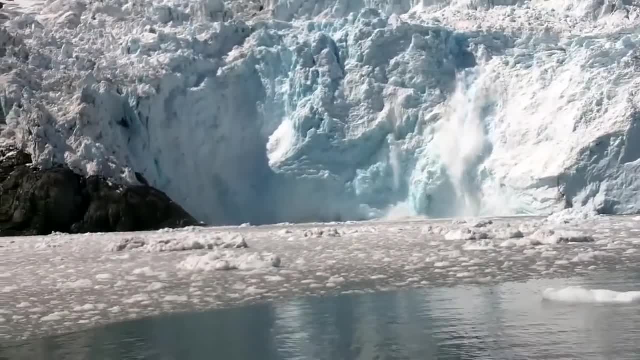 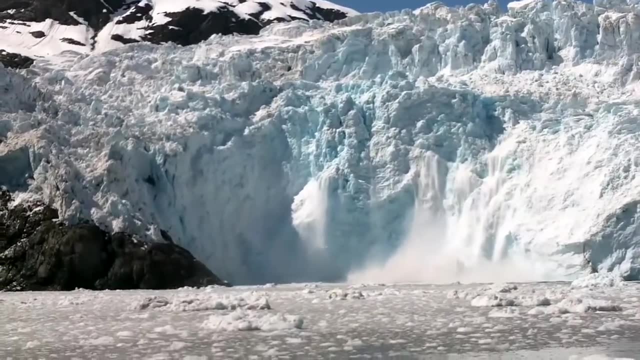 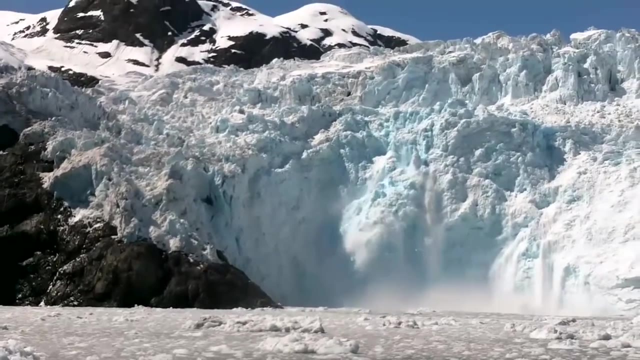 it forces the ice to retreat, forces the ice to melt down, break down and then to move, Moves down the hill. So I want you just to observe this: slowly but sure, It breaks down, disintegrates and then retreats. 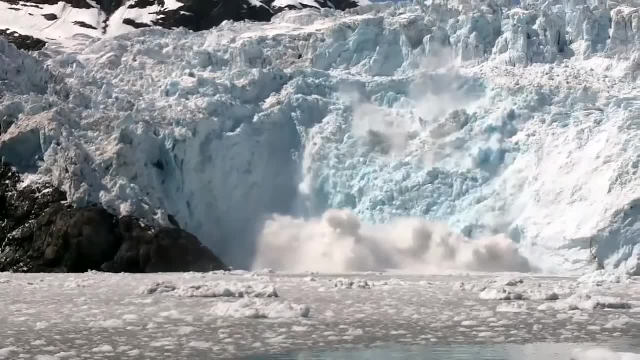 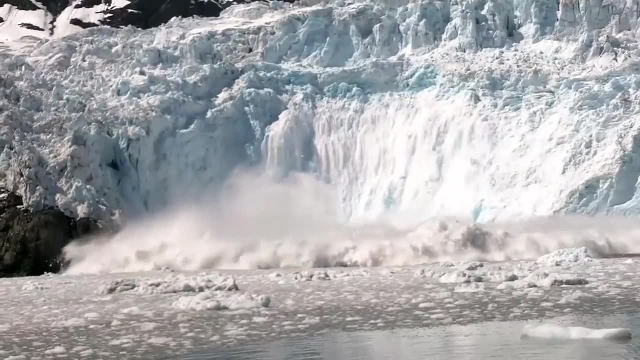 What you see there? you see massive, massive, my goodness, massive. What you see there is what we call carving of this ice. It's now carving in, It's retreating down the slope due to the massive weight and then the heat. 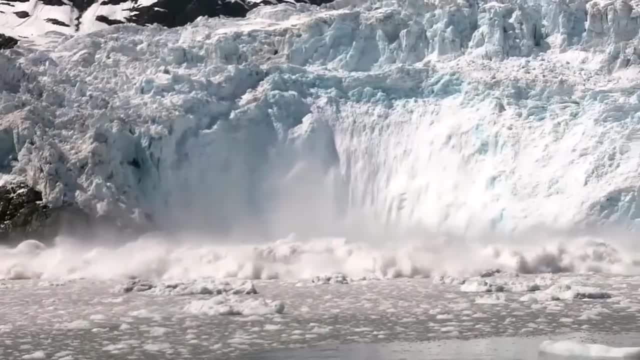 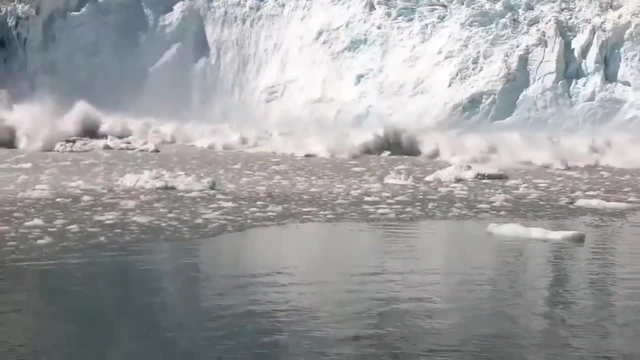 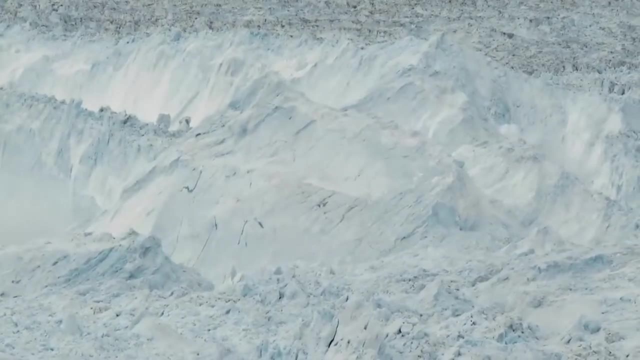 What you see. these are now summer conditions. These are the warm conditions that are forcing it to melt down and then move down the slope As it does. so we have seen earlier that it's doing what we call erosion. It is eroding and forming different kind of features that we have already seen. 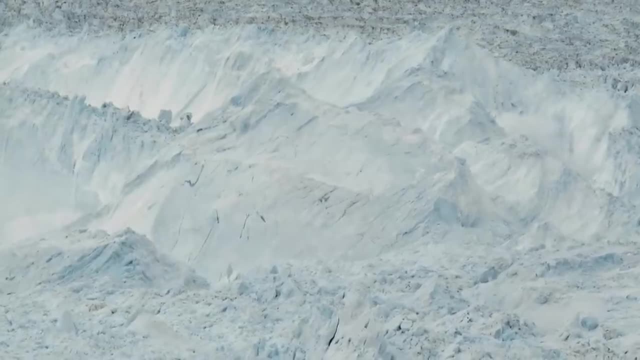 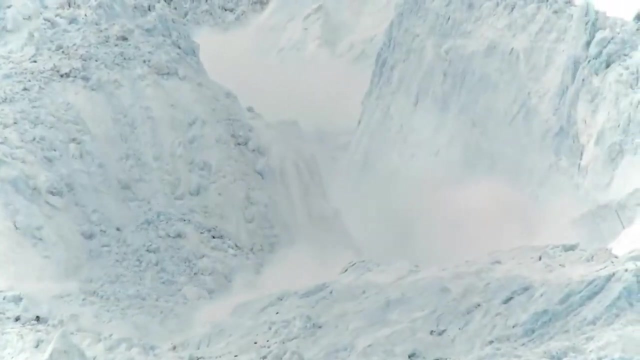 Right here also, we see a massive glacier. It starts slowly. With the time it will move massively. you can see there It is retreating down downwards. What you see there, please, it's not water. That's not water. 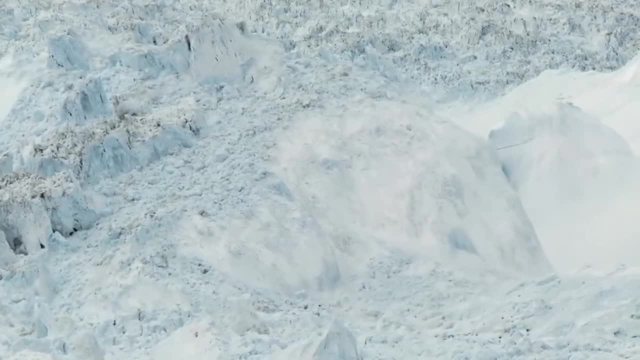 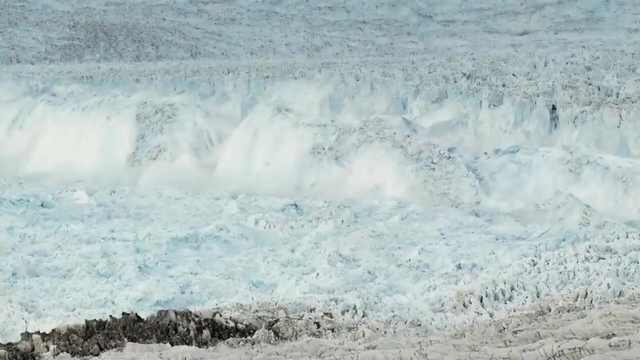 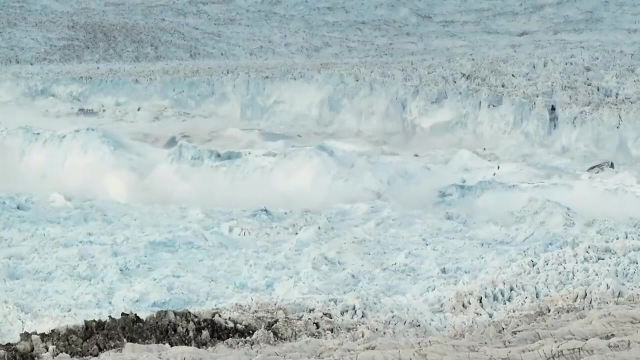 That is as simple as ice. That's ice rock that you see there And that's the massive glacier that we've been talking about. So it is retreating due to the warm conditions, and then the weight of it forces it to move beneath the slope. 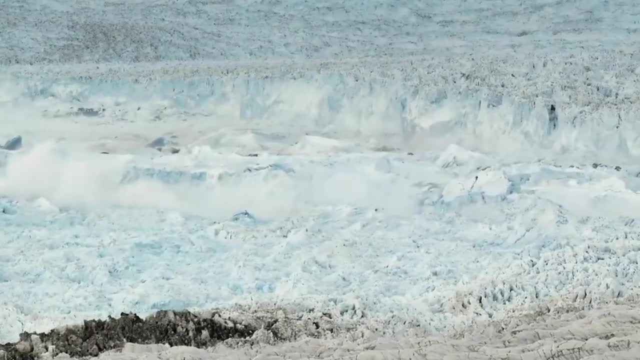 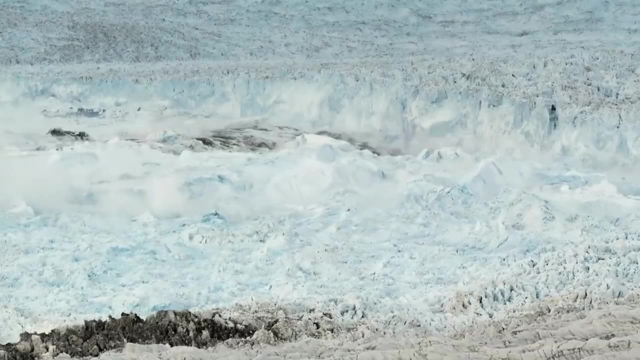 What we see there. it is doing a retreating and it is moving. That's the movement of this glacier, early alone, that we have seen. So it's massive, As you can see, very massive, And it's interesting right there. 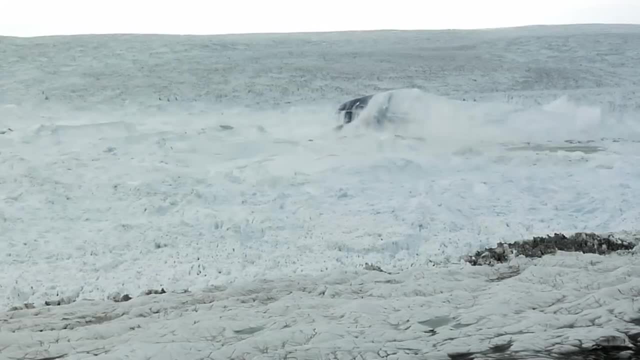 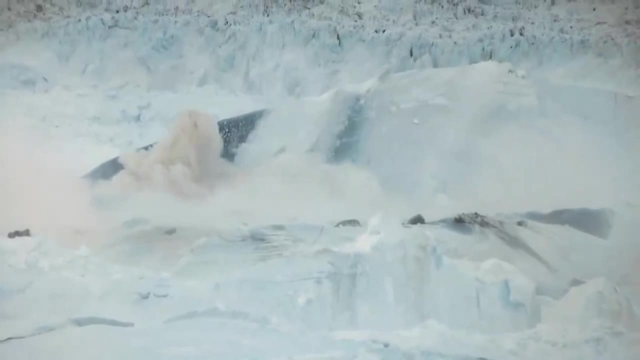 And that's how it does its process. With the time, it forms all the features that we have talked about. What you see, there is an ice sheet, That's an ice rock. that you see there, It's not water, It's not anything. 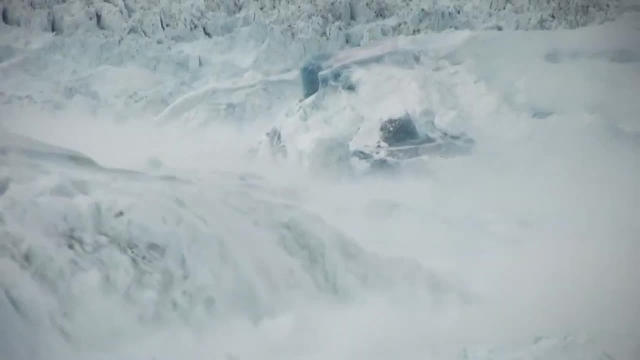 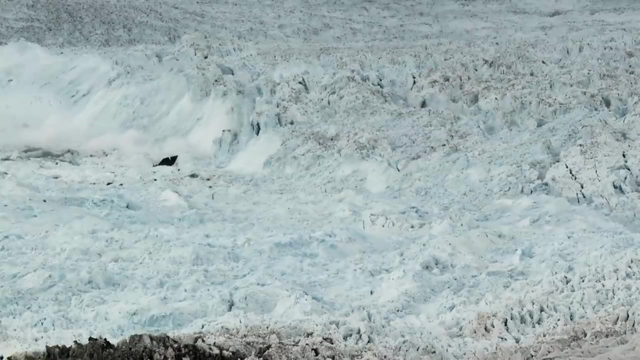 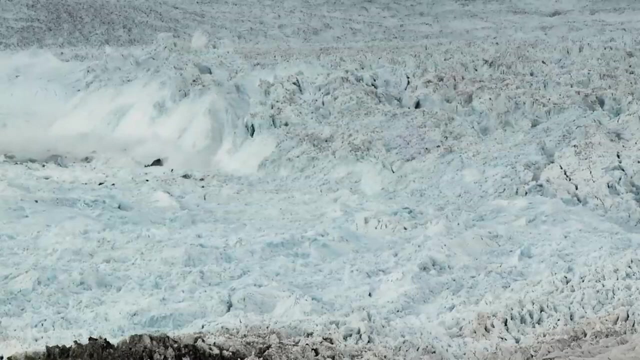 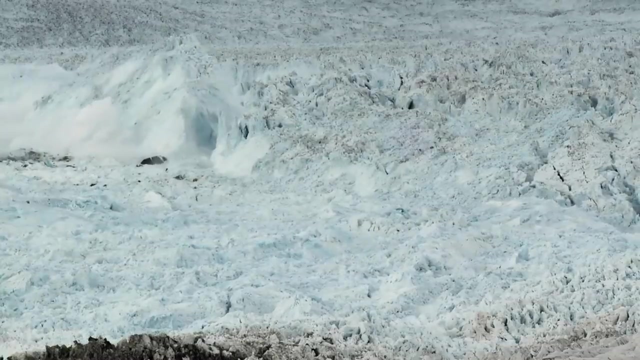 That is a glacier retreating, Basically ice retreating, as you can see right there. Quite interesting, Quite interesting. Keep watching, Just observe what is happening right there. It's because of what we have just talked about: The temperature is increasing and then the massive weight of this forces the glacier to move, to move, to move. 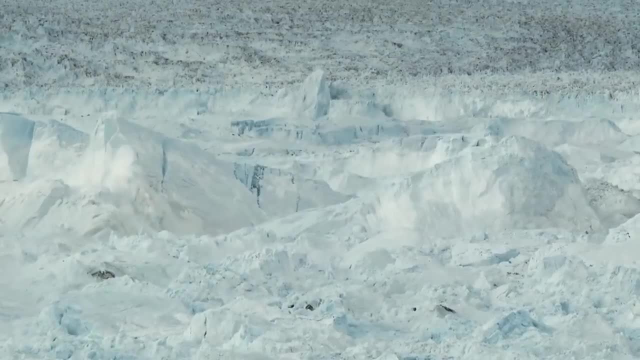 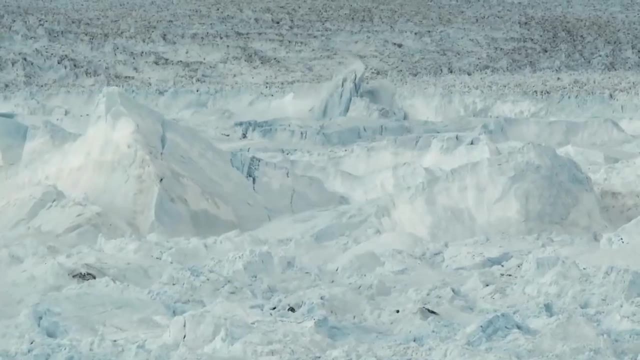 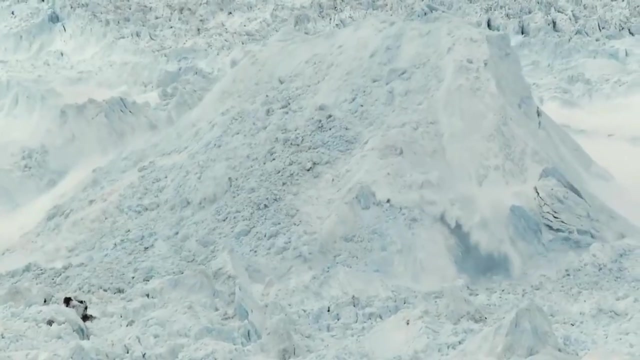 Retreating down the slope Right there. So you can see that is a rock ice there. It's a rock ice there moving And it's quite massive What we can see. there is a large area of this ice moving Moving. 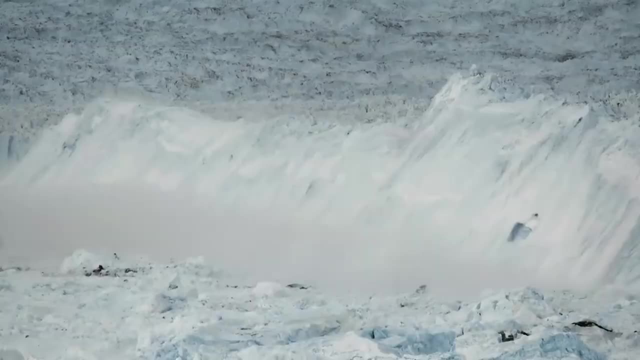 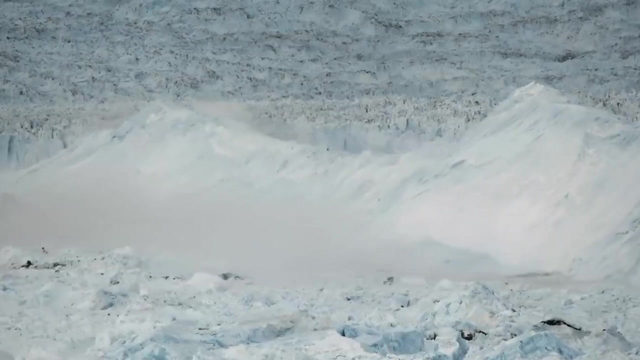 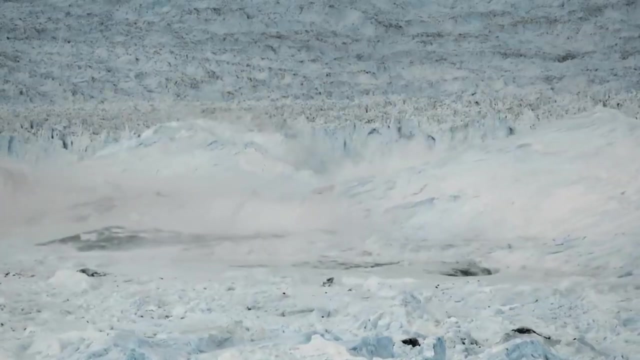 Right there, That is ice Moving from one place to another, And doing that is doing the processes of erosion and then deposition. I want to thank you so much for having been a good audience. We shall start from there. Please see you next time. Bye Bye, Bye, Bye, Bye.